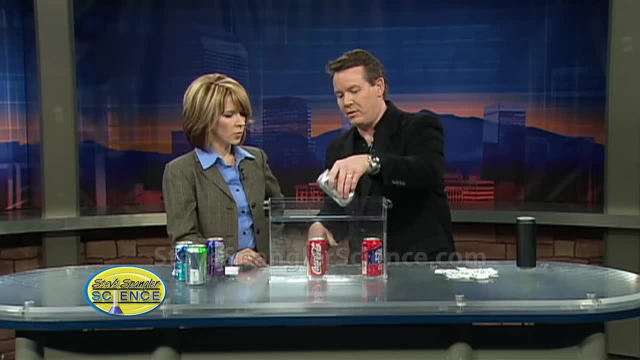 355 milliliters for a sink. A sink, Absolutely, So that one will sink as well. And then, if we try the Diet Pepsi, wow, there must be an air bubble. That's what it is: There's an air bubble. 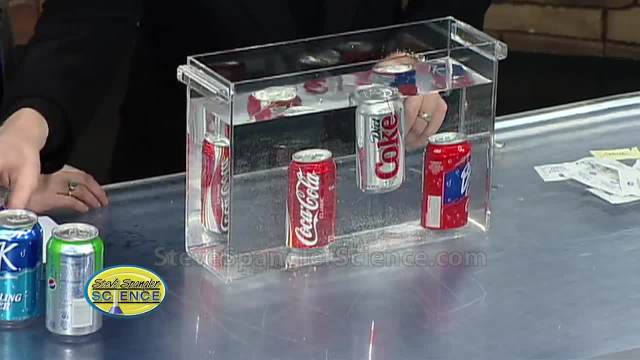 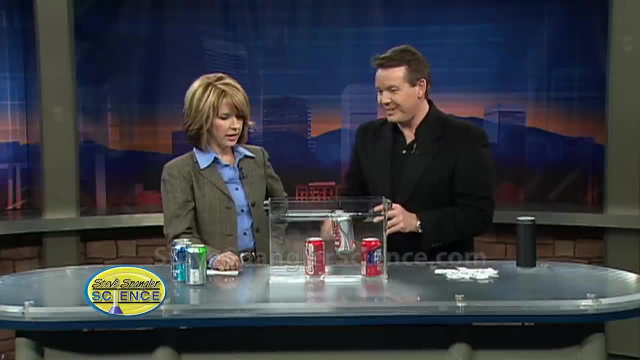 and oh my gosh, Wait just a second, Kim. out of all these here, which one's gonna float, which one's gonna sink? There's a Diet Pepsi, there's a sparkling water and a grape. Which one's gonna float? Well then, I'm going with the diet. Let's go for it, Okay. 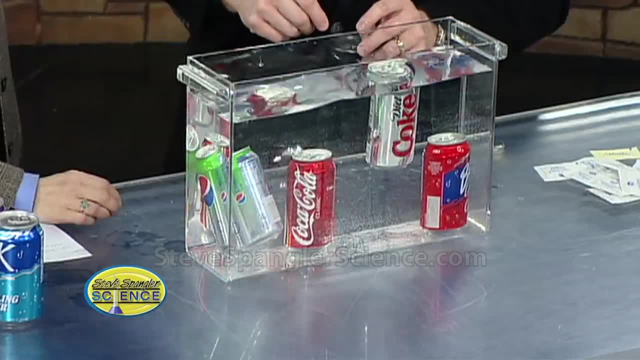 drop it right in there and see if you're there. It is, That's just. is it Okay? How amazing is that? Isn't that kind of fun? Now, there's not air bubbles underneath there, It really is floating. 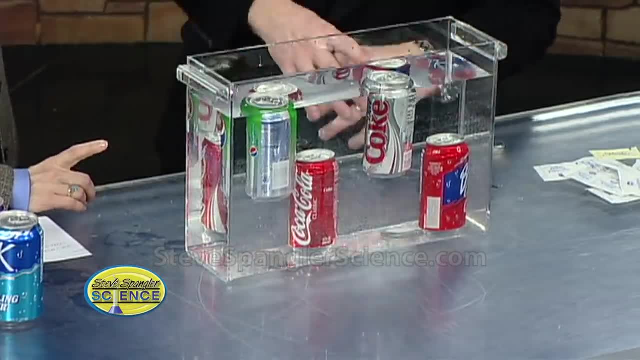 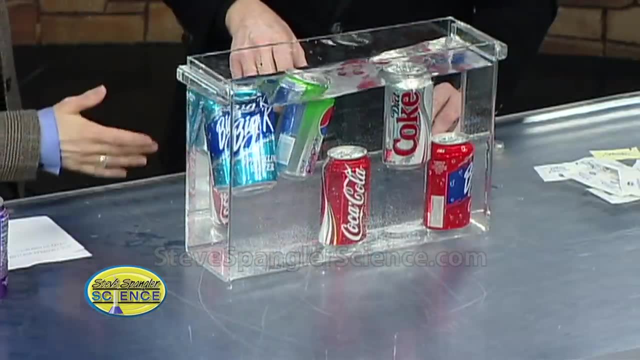 And so the general rule here is that everything that's diet will float, Everything that's regular will sink, Sink. So try that sparkling water. That's what I want to know, Just to see if that's there, you go, float or sink And we get a little floating action. that's there. So what's the? 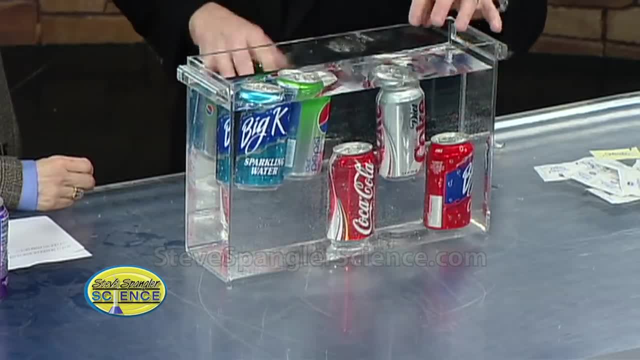 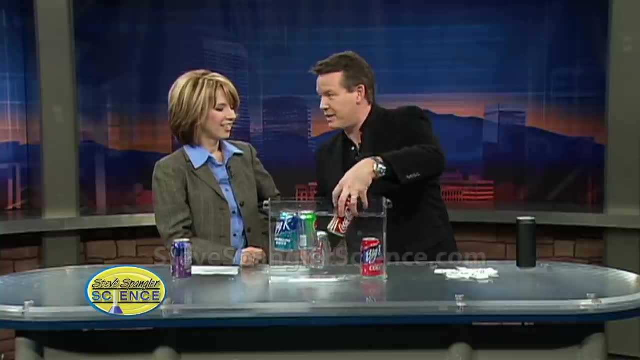 difference. And I asked a group of fourth graders what's the difference? Little girl, in all honesty, says it's the calories. This has 150 calories and this has no calories at all. And calories don't really weigh anything, except for the holidays, And they do. What's the big? 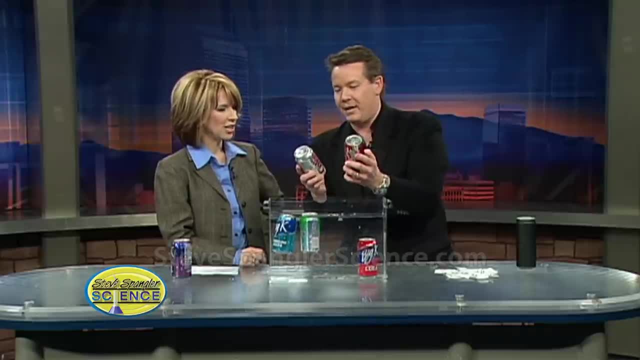 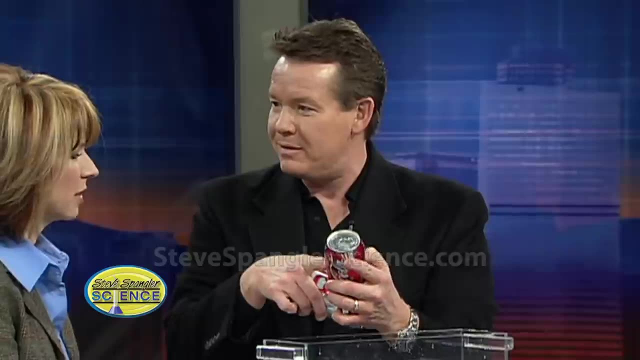 difference between the two. If you look at the difference, It's gotta be the sugar. Got it Right? So how much sugar in here? I don't know A lot of sugar. 39 grams of sugar. But you know why they put it in grams? Why, Because we're Americans and we don't get that. Yeah, because 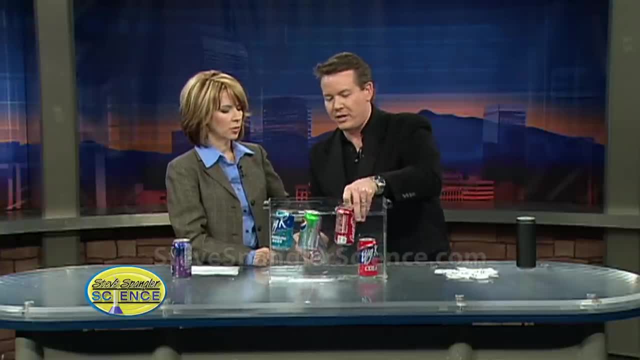 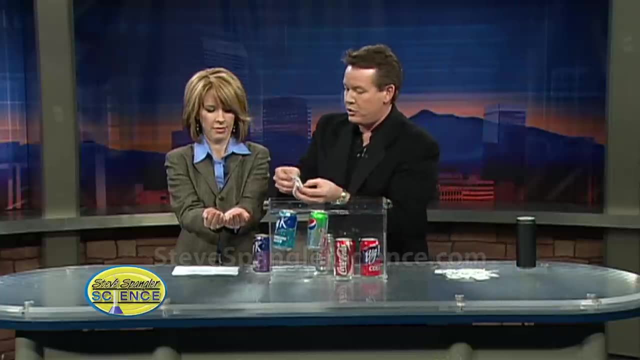 it means nothing to me. 39 grams must be nothing, right? So how much is 39 grams? Well, I think maybe the best equivalent is for here: Hold out your hands right here. I'm going to put packets of sugar in your hands. You tell me when to stop. All right, So here we go. One, two, three, four. 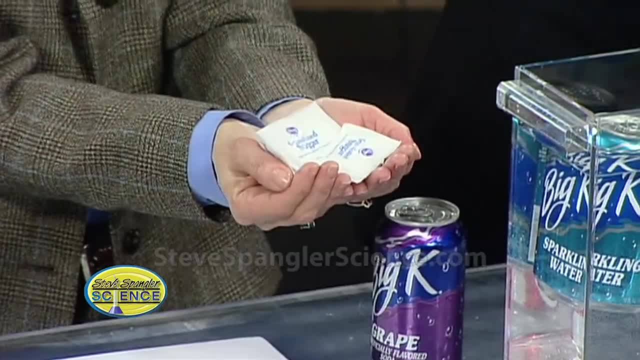 More than that, I'm thinking more. Okay, Five, six, seven, You tell me when to stop. Eight, nine, Oh, that's enough. Okay, Keep going 10.. Keep going. 11,, 12.. You want to stop? Yeah, No 13,. 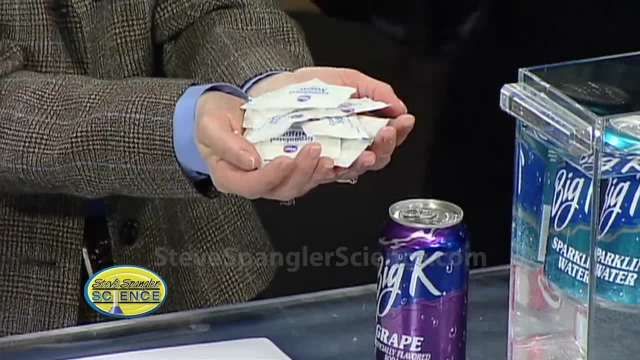 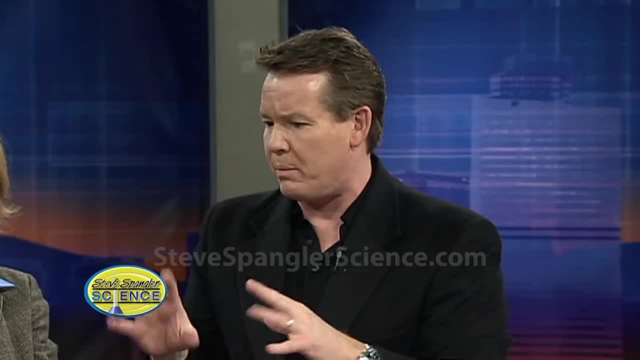 14,, 15,, 16,, 17,, 18.. Roughly 18 packets of sugar in that Coke that you see down there. Now we've taken some liberties because there's high fructose syrup, And so about 18 packets of sugar, That's. 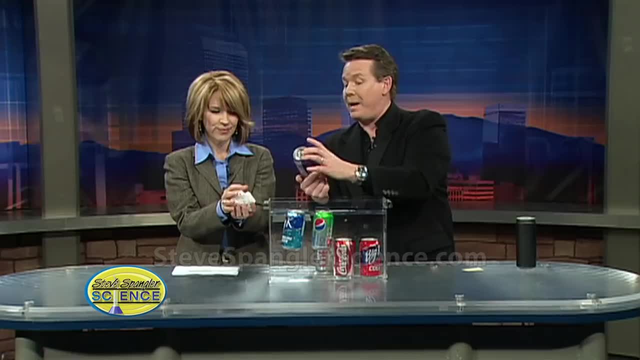 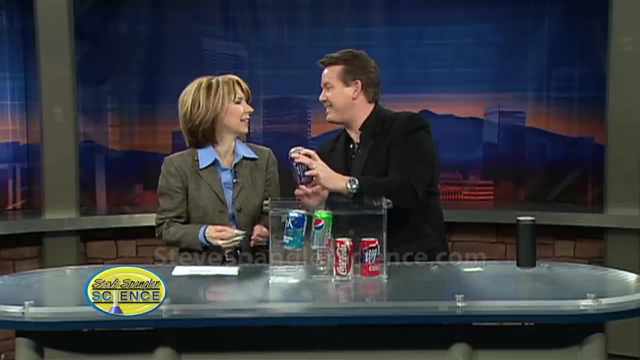 only 39 grams. Take a look at this guy over here. This is grape soda, So this is going to be really good for you. How many grams Right there? Oh, 14.. No, 60.. I can't see, It's okay, I'm sorry. 54.. 54.. Watch this thing.